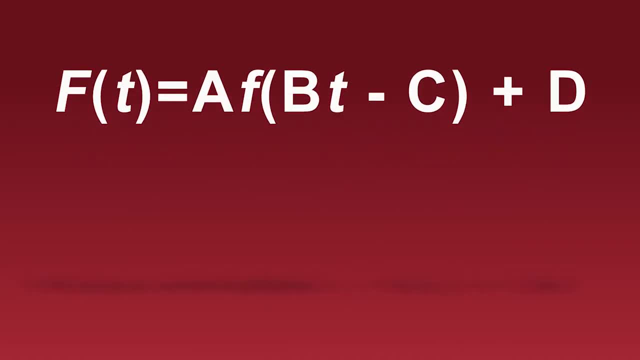 function To begin shifting trigonometric functions. write the trigonometric function in a specific manner. By writing the function in this format, we can easily identify the components of a phase shift or vertical shift. F of T represents the trigonometric function. A represents the amplitude of the function. 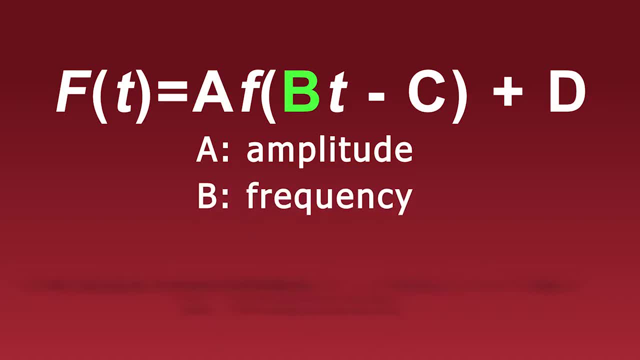 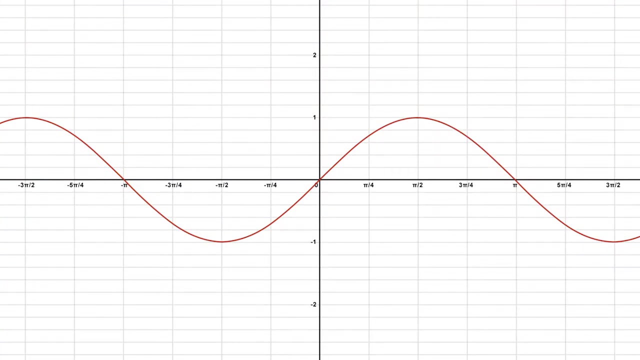 B represents the frequency of the function. C represents the phase shift of the function. D represents the vertical shift of the function. For this specific concept, we will focus on the components C and D. Let's take a closer look at each of these components. For the phase shift, the constant C moves the function to the 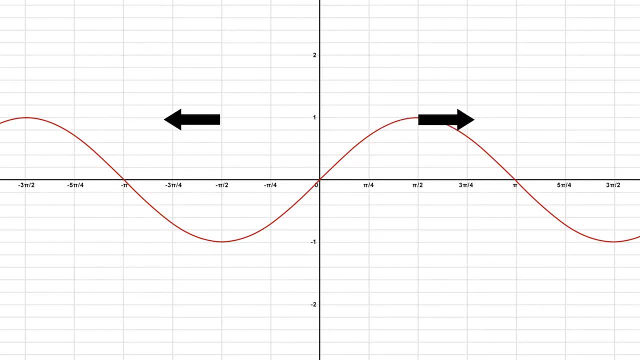 left or to the right. C units on the course. When the phase shift of the function is removed, the function moves a coordinate grid when b equals 1.. If the horizontal shift is positive, the function shifts to the right. If the horizontal shift is negative, the function shifts to the left. Note that: 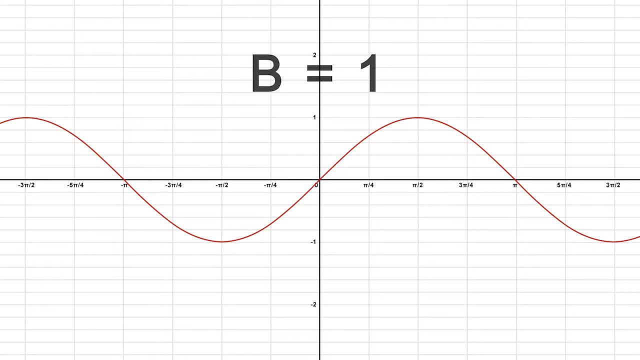 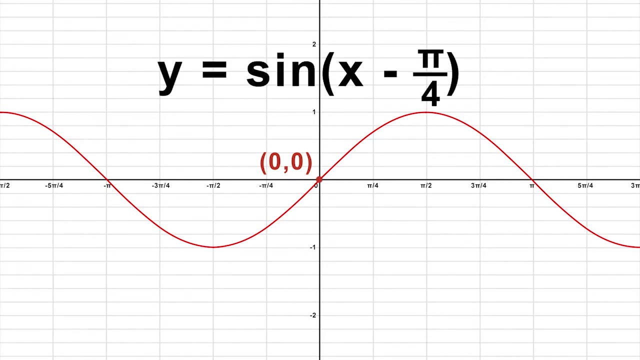 this occurs only when b equals 1.. This is the basic sine function, which is represented by the function y equals sine of x. If we are given the function y equals sine of the quantity x minus pi over 4, the function on the screen c equals pi over 4.. Since pi over 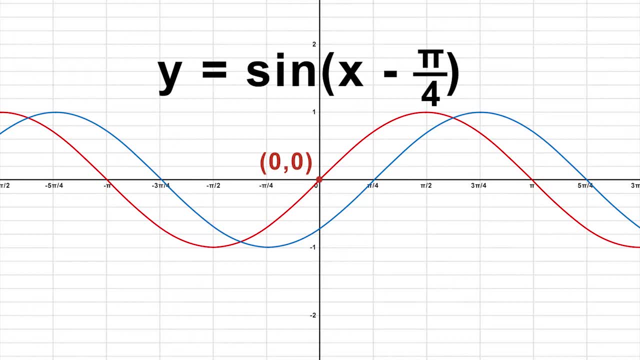 4 is positive, the sine function shifts to the right pi over 4 units. This means that the graph of this function shifts pi over 4 to the right. Let's look at another example. This picture represents the basic cosine function. This: 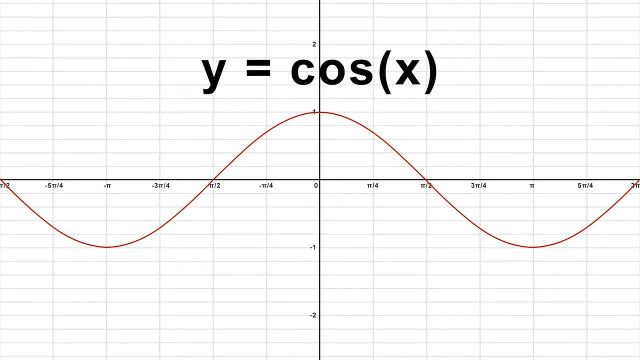 function is represented by the function given, which is: y equals cosine of x. In the function, y equals cosine of the quantity x plus pi over 2, c equals negative pi over 2.. We have to rewrite this function. Let's rewrite the function in the same format as the basic function. Rewrite the function.